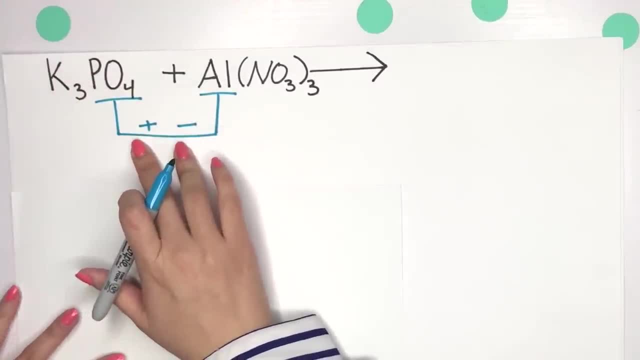 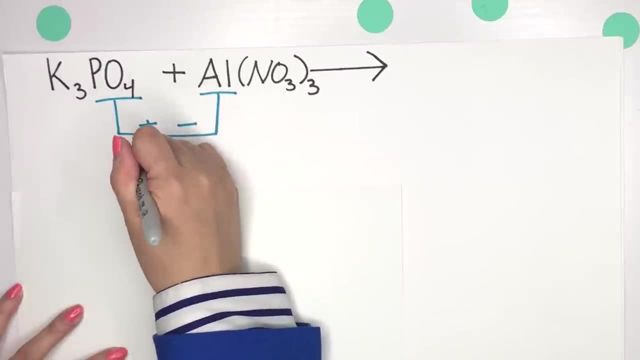 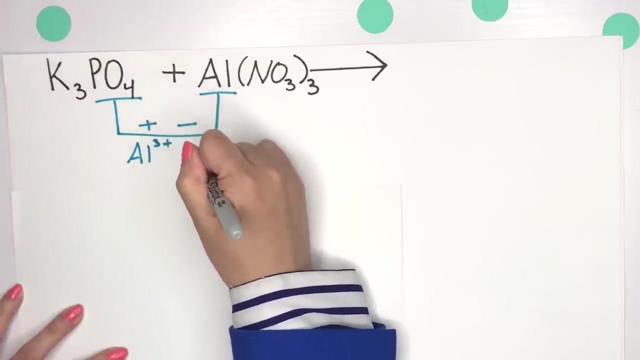 negative. This is going back to also an ionic compound, where we have a metal that's positively charged combined with a non-metal that's negatively charged. So aluminum has a three plus charge, and phosphate, one of our polyatomic atoms, has a three minus charge. So, luckily, 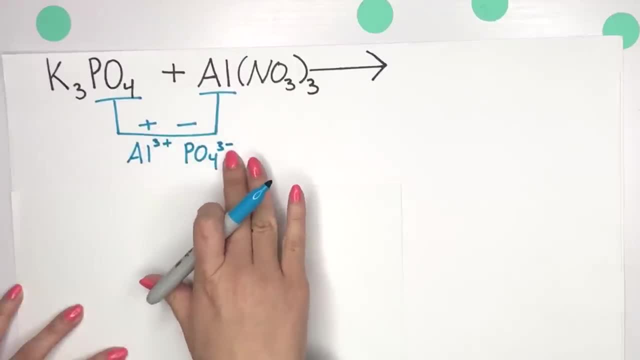 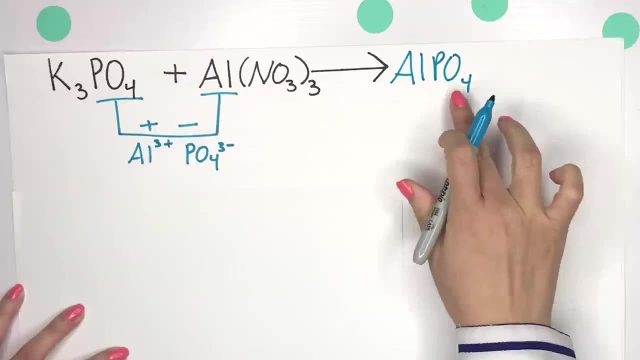 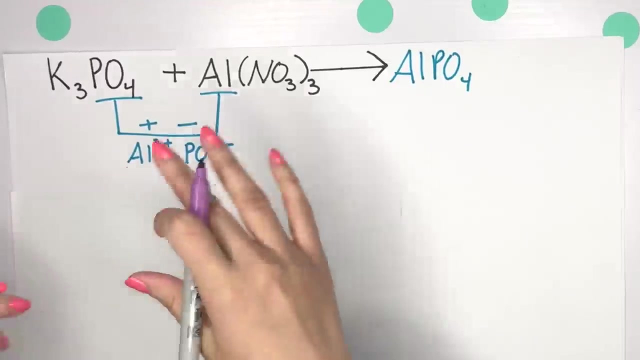 right then, and there that's completely balanced for our charges. So our first product- we don't have to add any other subscript, and it's just aluminum and phosphate. That's the inner with the inner. Now let's look at our outer with our outer. So our outer with our outer. 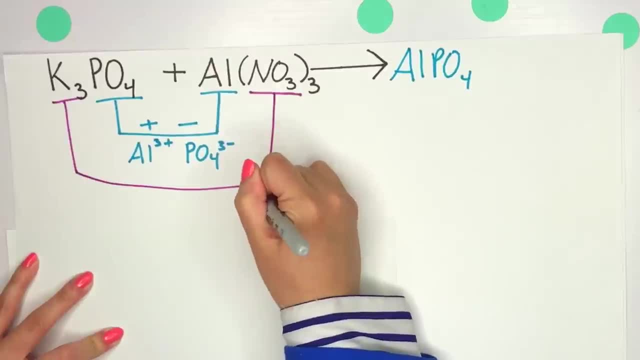 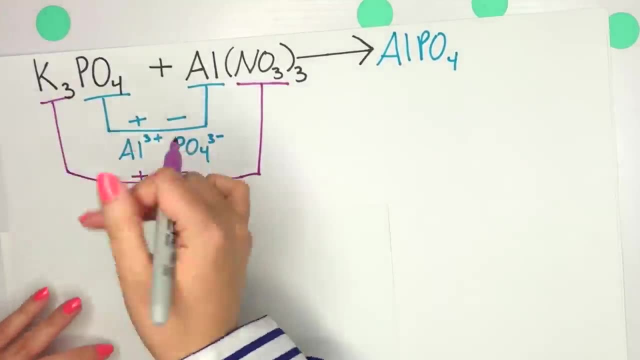 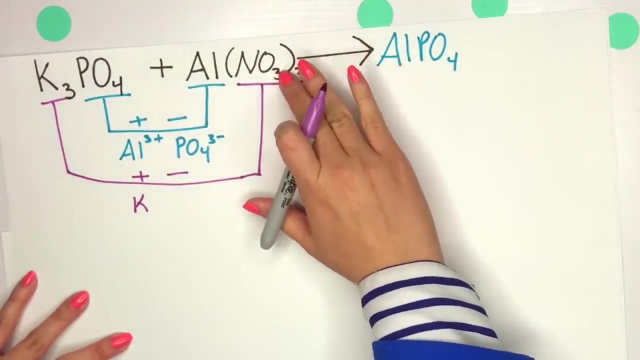 will combine these two to form our next product, our next compound, always thinking positive before we think negative. And we're going to put that potassium first, since that is our metal and that's our positive charge, And then it will be followed by nitrate, since that's our negative charge. So potassium has a plus one charge and 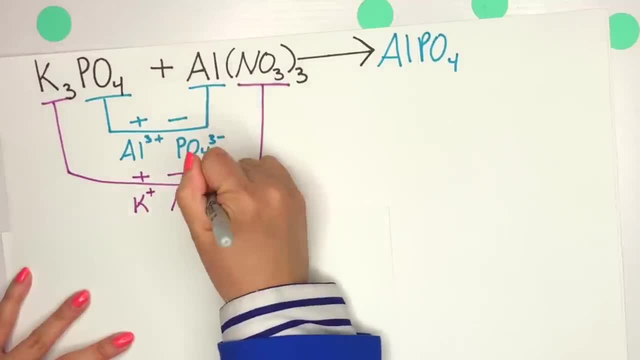 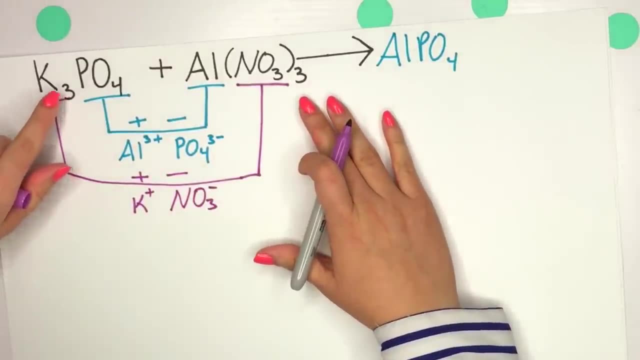 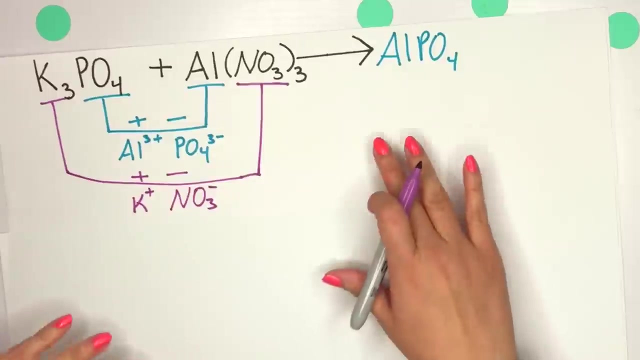 nitrate or NO3 has a negative one charge. Note that I did not bring this subscript, that three, on down because that three was only there to balance out the charges within potassium within this compound as a whole. Same thing with this other subscript of three for nitrate. I did not bring that down. 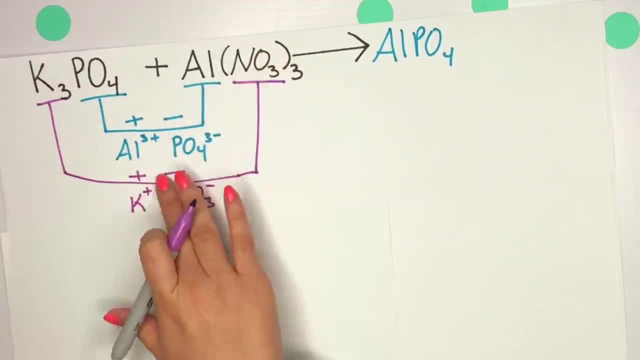 This is a totally different three. Right, I took that three from O3, because that's just what our polyatomic atom is. So these other substrates do not come down when you're predicting your products now. continuing with this, our charges are completely balanced. 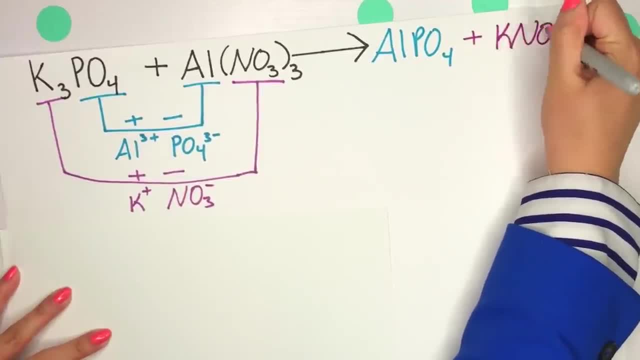 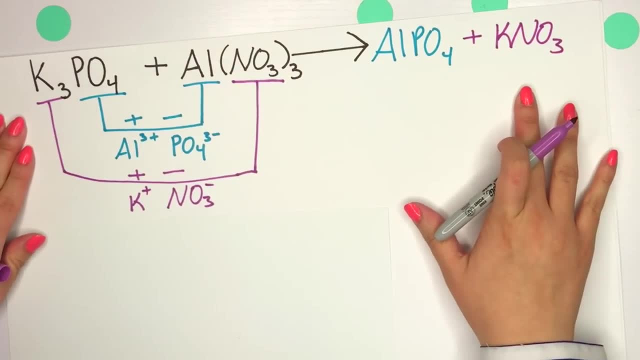 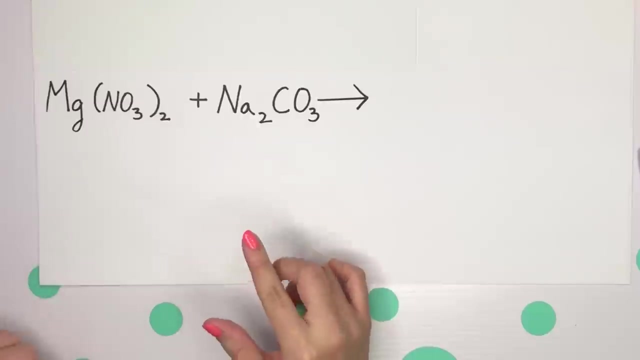 So we will get our next product of potassium nitrate. note that I have not balanced this out, actually not going to be balancing equations right now, just showing you how to predict products as a whole. Let's try another example with that whole: inner with the inner and outer with our outer. to